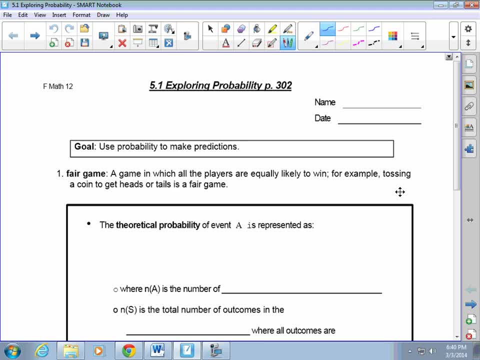 Chapter 5 is. unit is on probability and with the probability we're going to be using some of what you've done already in your last two units with our last minute odds and and things like that. everyone we're doing our sets, not our odds, our sets probabilities, looking at odds, so you'll see some overlap of what you've. 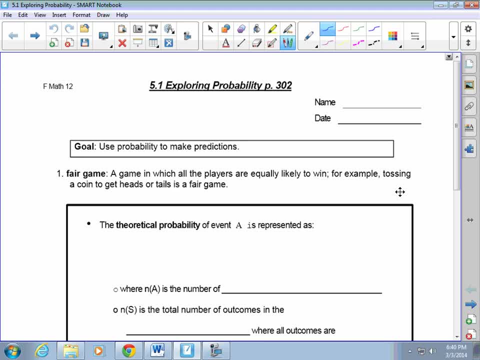 done in the last two chapters, and little bits and pieces will be popping up here. so what we're looking at in this first section is exploring probability, just basically finding out what it means and what do we do with probability. the goal, then, is to use probability to make predictions. so we've done in the first 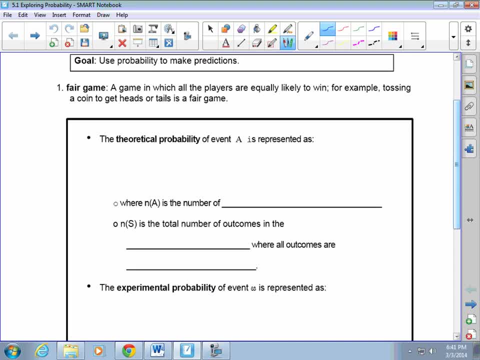 chapter there where you were doing the converse and the inverse and conditional. those things are going to come up a little bit in in what we're doing here. so first thing is a definition of a fair game. so a game, a fair game, is a game in which all the players are equally likely to win. for 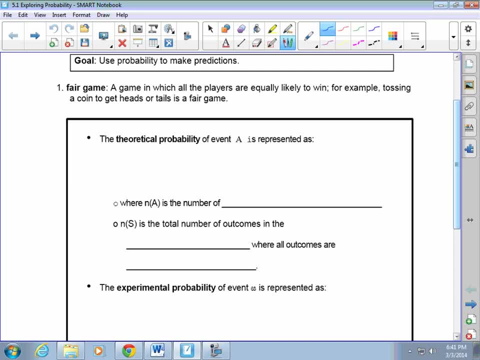 example, tossing a coin get heads or tails is a fair game. so an unfair game would be if you had a coin that was fixed and it had both heads or both tails. so theoretical probability of event A is represented as probability of A and probability is always a capital. B is equal to the number of things or number. 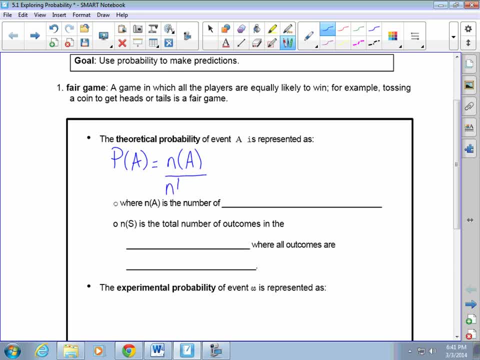 of elements in A over the number of elements in S, where NA is the number of favorable outcomes for event A, so favorable outcomes means that that can happen. and number of elements of S is the total number of elements, so there is a total number of outcomes in the sample space S, where all outcomes are equally. 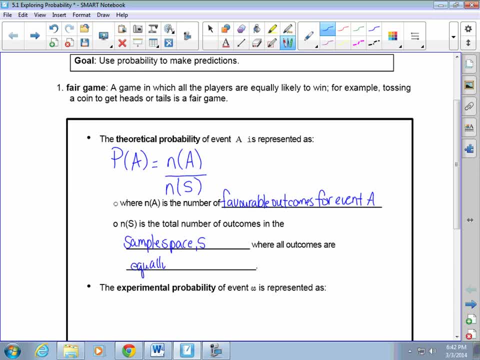 likely. so that's saying you would have a fair base or a fair coin or two деревmo, and in other words, all that is scary, a fair game. So that's theoretical probabilities. a number of favorable comes over all the number of possible outcomes. experimental. 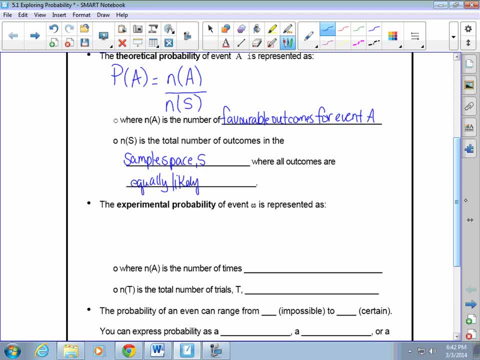 probability of event A. have an event and that should be a. there- my smartboard copy didn't do that well- is represented as the probability of a is equal to the number of A over number in T, So where number of A is the number of times the event A occurred. so 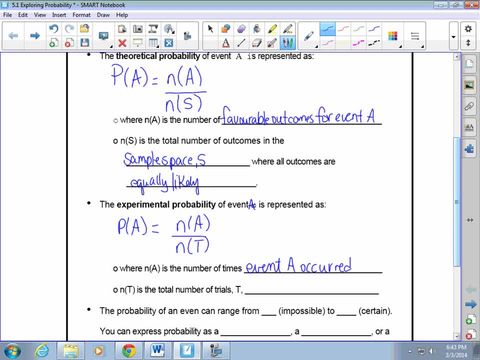 that it actually happened, and N of T is the total number of trials- T in the experiment. So excuse me, experimental probability- then you're basing it on how many times it took you to get the number you were looking for. So if you're trying to get 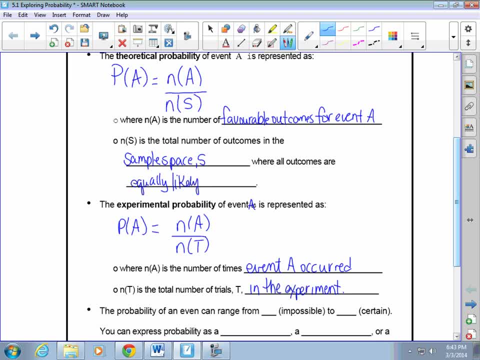 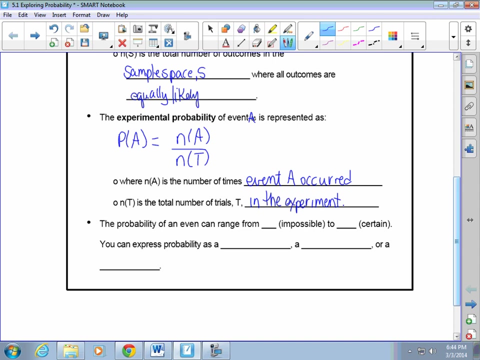 nine tails on a coin. but how many times did it take you to get nine tails Okay, so that your number T would be: maybe you had to flip the coin 25 times in order to get that. Probability of an even can range from 0,, which would be an event, can range from 0, so you can't get it all to 1, and that means it's a certain event. 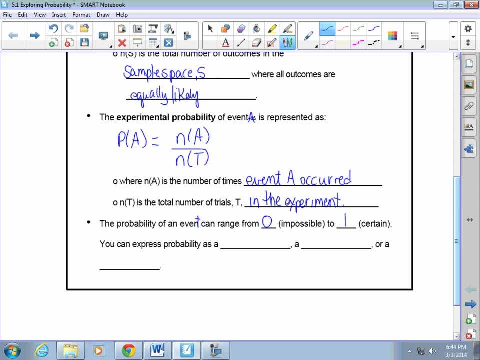 You can get it, no matter what You can express probability- as a fraction, a decimal or as a percent. So the probability of an event happening is always going to be between 0 and 1.. 0 means it's impossible to get that. 1 means you're certain to get that. 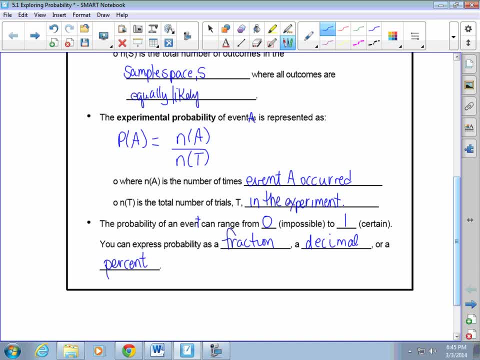 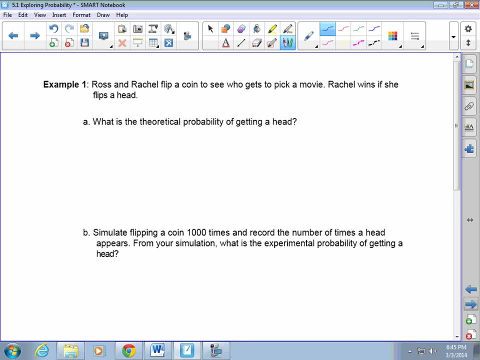 So let's try to put these two probabilities, theoretical and experimental, into action. So let's say that we need to put this one into action. It says Ross and Rachel flip the coin to see who gets to pick a movie. Rachel wins if she flips a head. 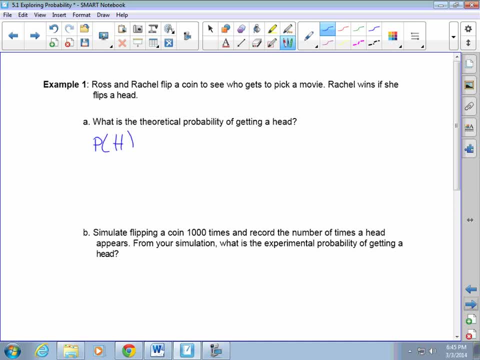 What is the theoretical probability of getting a head? The probability of getting a head she just wants to get. remember the number in A over the number in the sample set. So the number in our sample set is: do they get heads or tails? Well, do we look at that? Of course we do, And I am going to get a head. Now. how many tails are there? One, two, three, four. Everybody is asking for A. Who's getting A? 20% is going to get A. 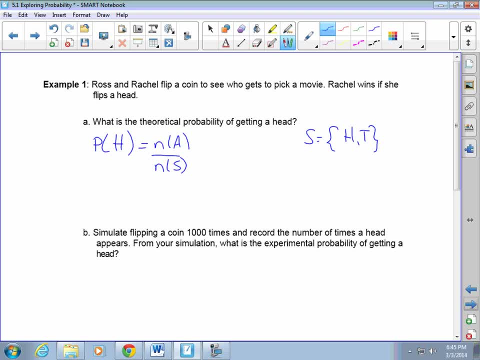 40% is going to get A. That's the number in the sample set. So where can this one be? 20% is going to get A. looking for We're looking for. where does she have to get The head? So that means 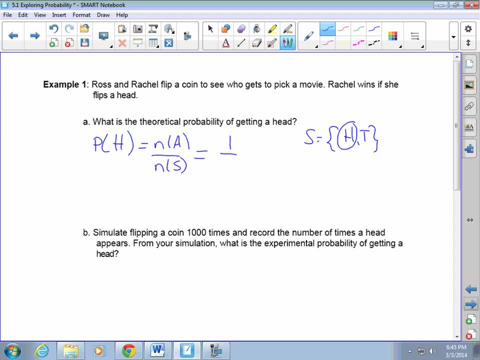 number of events. where that occurs, favorable outcomes for that event is one. number in the sample set is two. So it's a half, 0.5, or 50% chance that she's going to get the outcome she wants. Simulate flipping the coin 1,000 times. 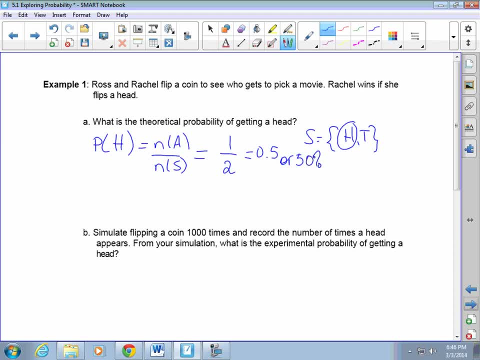 and record the number of times a head appears From your simulation. what is the experimental probability of getting a head? So what you can do is you can actually go, and I'm not going to go on there, but you can go on to if you just. 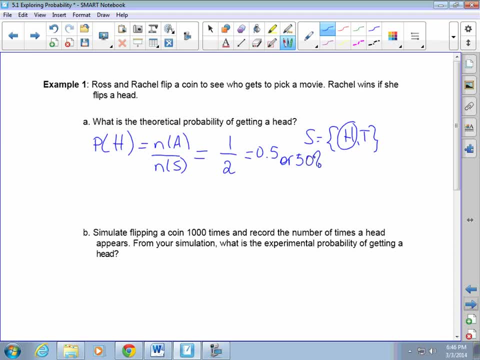 google it and do coin toss simulation and you can put in there how many flips you want and you'll pick your, you'll enter in a thousand and then it'll just do it for you and it'll come up with a number. So I did this beforehand and the 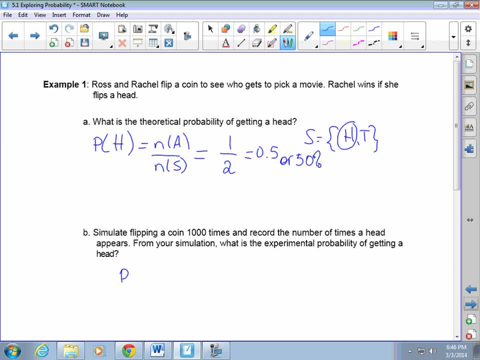 one that I got was probability of getting a head. so this is in experimental. so that's the number of A over the number of trials. So we know our number of trials in the experiment was 1,000, and in the simulation that I did there were 484 heads. that happened in. 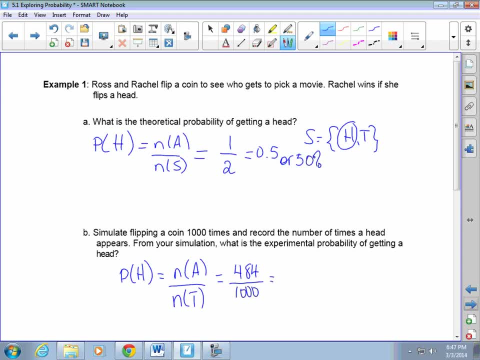 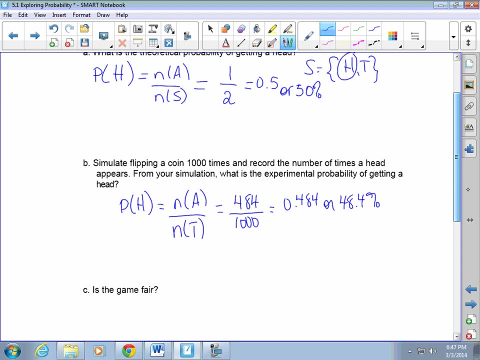 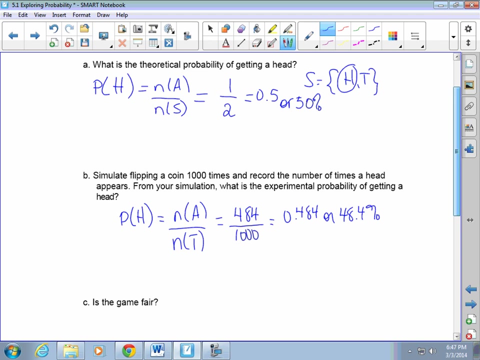 1,000 tosses, So that would be 0.484, or 0.484%. So CPart says: is the game fair? Well, remember to be fair. all the outcomes have to be equally likely. so this would be a fair game, assuming that you have a coin. 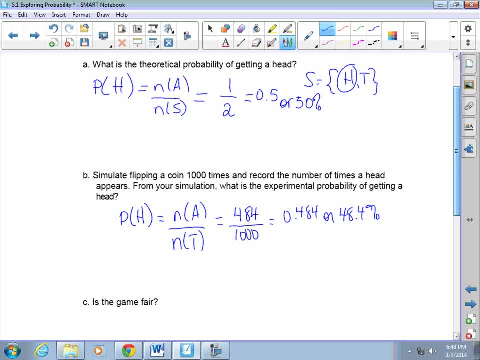 that's got heads and tails on it, So it's a fair game because of that, because you, each outcome is a fair game, equally likely, Okay. so in that, the one flip of a coin, you see that she has a 50% chance doing 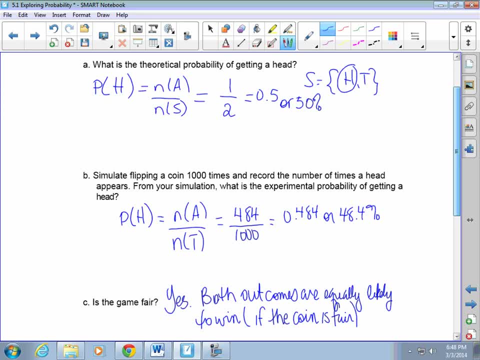 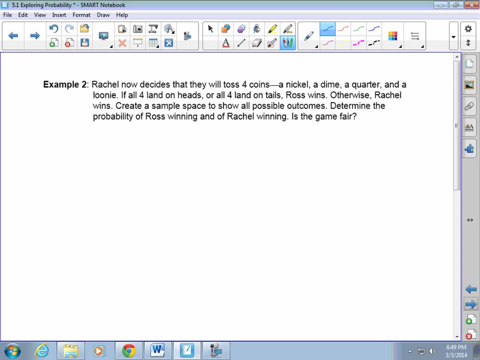 it a thousand times. it was pretty close to that 50%. it was just 1.6% off of that 50%. Okay, it says. Rachel now decides that they will toss four coins- a nickel, a dime and a quarter and a loonie, if all four land on heads or all four land on tails. 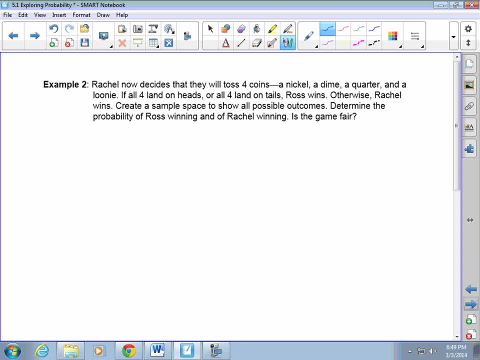 Ross wins, otherwise Rachel wins. Create a sample space to show all possible outcomes, Determine the probability of Ross winning and of Rachel winning, and is the game fair? Okay, so we need to have. She's got a nickel, a dime, a quarter and a loonie. 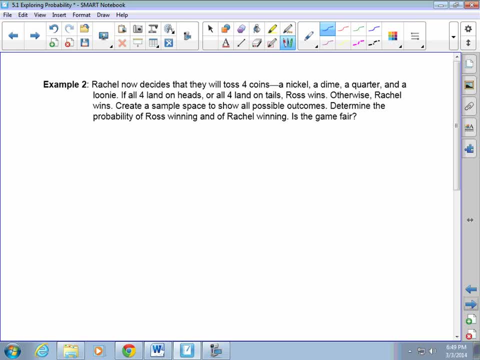 So the first one that she tosses- whichever one we can say- it's the nickel. so she's got 0.5% chance of getting heads and 0.5% chance of getting tails. Okay, Okay, Okay Okay. 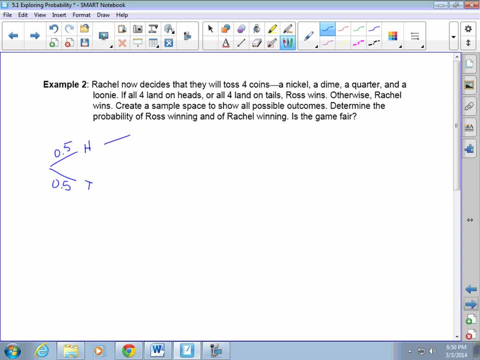 Okay, Okay, Okay. Oh, that's a nice one. She's got a coin, We've got our heads and our tails, So she'd have 0.5% there, 0.5% there. If it had been a tails, than that coin toss would have been 0.5 or 0.5 for heads or tails. 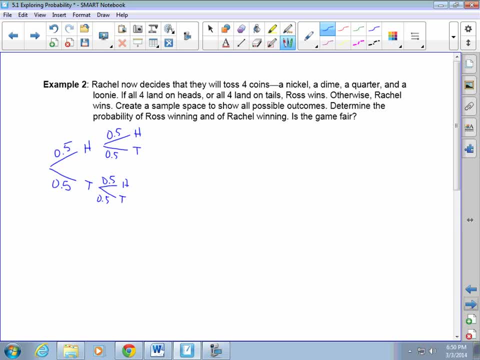 So then, from this coin toss, if they had done, if they'd have done- I'm going to be, I've started this a little bit high- Heads and tails again 0.5, 0.5. So after this one it could have been heads or tails at 0.5 and 0.5. This one would 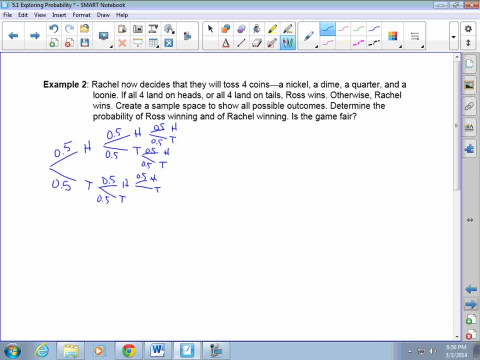 have been heads or tails, the next coin- oh, I can't say that coin toss. And then if this, that coin toss, had been a tails, then the next one could have been heads or tails. So that's three coin tosses. So now we have to do it for the fourth coin toss. 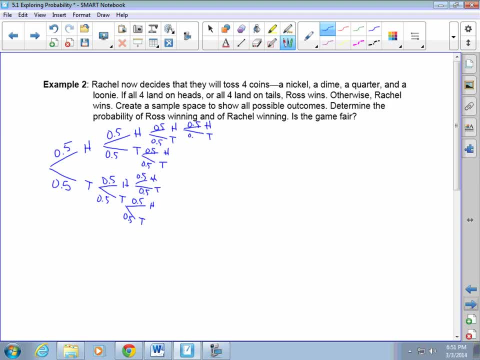 So heads or tails, 0.5 for each. I'm going to do this one kind of like this. So 0.5, 0.5 again This one. if they'd have tossed the coin, she could have got heads or tails. 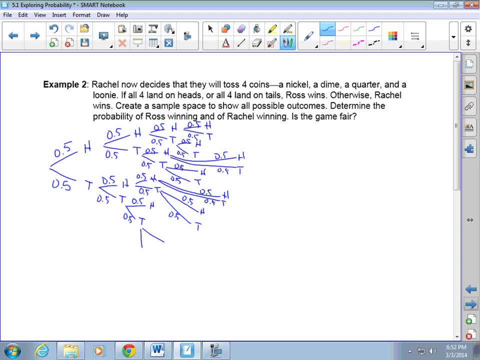 Okay. so then, on the last coin toss here, I'm going to do this one kind of like this. So I'm going to do this one kind of like this. I'm going to do this one kind of like this. So if I'd have done this actually a little bit lower, it would have been easier. 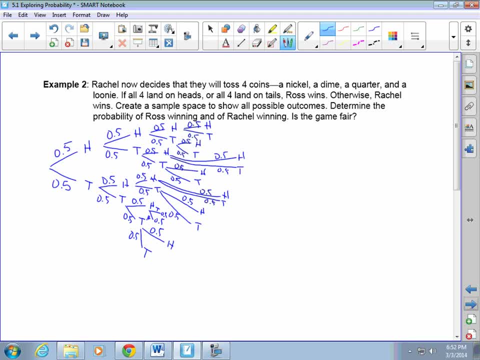 to see what I'm doing. This needed to be down, But the first coin, toss, could have had a heads or tails, so that would have been this one right here. So then the second coin, toss. if they tossed a heads, their next coin would have been heads or tails, But so that would have been. 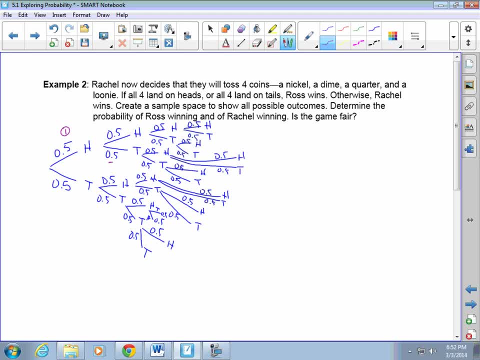 this one. But if they had tossed a tails, then the second coin toss could have been heads or tails. So that's why each of these branches out And then each of them for each possible outcome. then you have to do a heads or tails from there. So if we take a look at this, 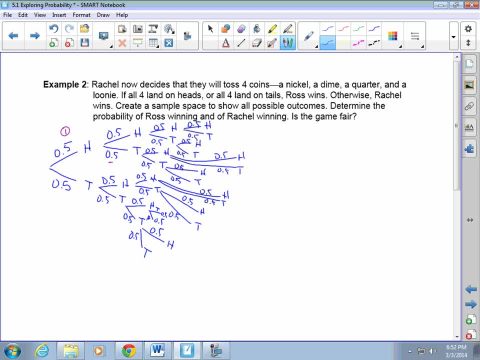 possibility of getting all heads we have. we've got head, head, head and head, So there was getting four heads. there was 0.5 times 0.5 times 0.5 times 0.5.. 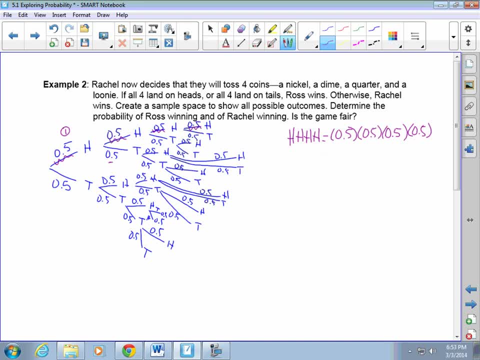 So that was the probability for each one of those. So that is equal to zero. if you multiply those together, 0.0625.. For the tail one: so that's, here's a tail, then lift a tail, lift a tail, and then the fourth flip of a tail, same thing: 0.5,. excuse me, four times. 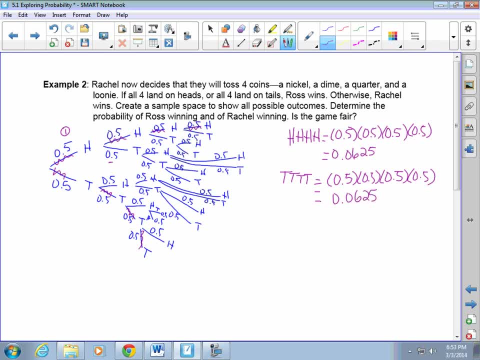 So that is equal to 0.0625.. So possibility of Ross winning is that 0.0625 plus 0.0625.. So that equals 0.125 or 12.5 percent. The probability of Rachel winning then, which we know. the total probability of winning is one. 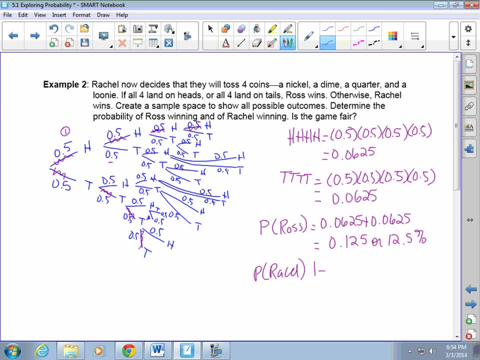 minus Ross's probability. So if you were to multiply everything else that's in here side here together, you would get this answer. But easier way to do it is to take Ross's away from the total number of probabilities. So one minus 0.125 would be 0.875 or 87.5 percent. 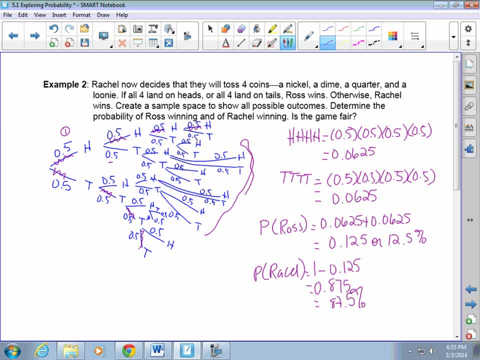 0.875 or 87.5 percent. 0.875 or 87.5 percent. So the probability of Ross winning and Rachel winning Ross winning is 12.5 percent, Rachel winning is 87.5.. Is the game fair? Well, no, The game is fixed because each outcome isn't. 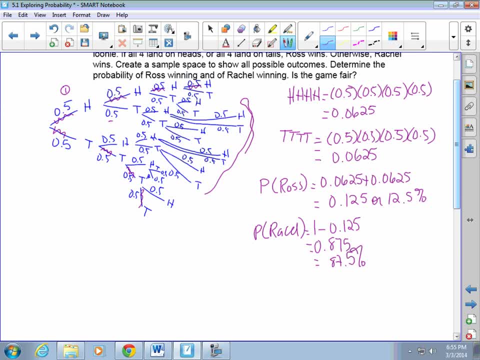 as equally as likely, because you've got a restriction on there for for Ross's, where he has to get all heads or all tails. But you know, I'm comfortably talking to myself on that, But there's the blinded building in between. They didn't win. So I'll муз the yanks all in back at you: one, two, three and one. So the game is fixed because Rachel has a better chance of winning. So the game is fixed because Rachel has a better chance of winning. 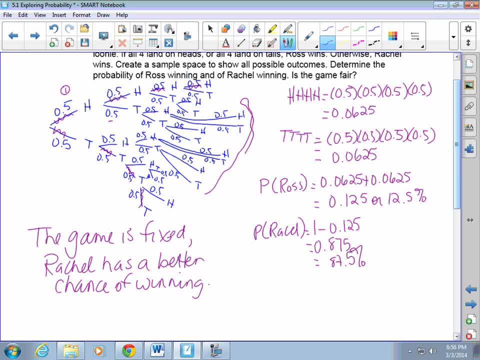 So when you're working on these questions, you just have to keep the, the two main formulas straight. one is theoretical. So when you're working on these questions, you just have to keep the, the two main formulas straight. one is theoretical probability- the normal sai to mo- for RayTal's, and that's using the number and the example. 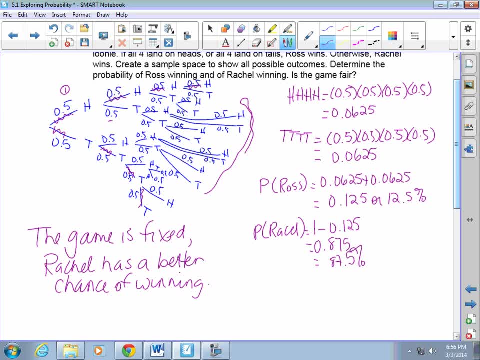 and that's using the number and the sample set. so the number of outcomes that you're looking for over the number possible in the sample set. so if it's a dice roll, the number of possible in the sample set a regular dice would be six and if you're looking at coins, your 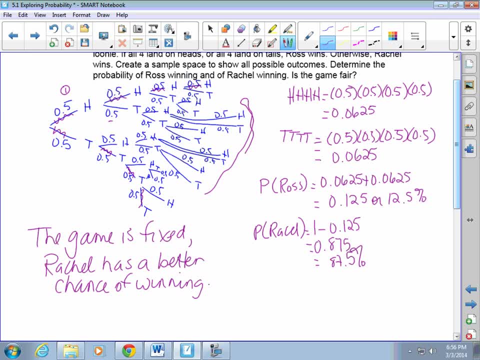 number in the sample set would be two. you'd have heads or tails. if it's a deck of cards, it's 52, or if you're looking at certain suits, then it would be in 13s. so that's theoretical probabilities. the number in the sample set: experimental. 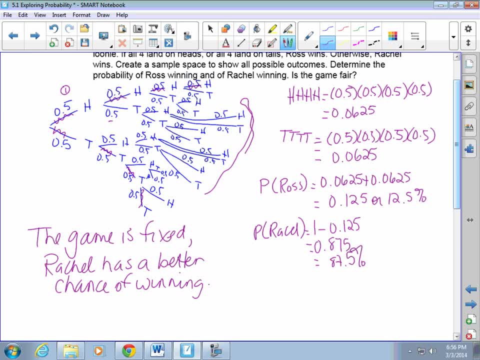 probability is when you're trying to see how many outcomes you can get in a set number of trials. so your trials are what you keep track of and then the outcomes that you get. so if you're rolling a dice a thousand times, that would be your number of trials and if the outcome you're looking for is a one, 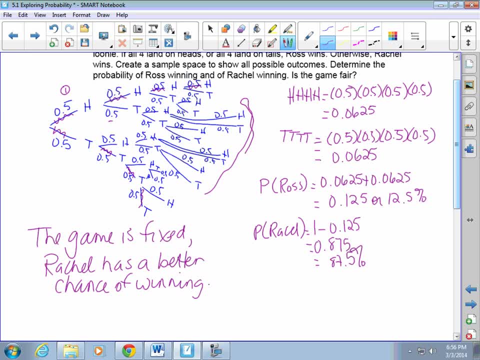 or a three, then you keep track of. okay, I've rolled the dice however many times, a thousand times, and I've got three, threes, which you should have more than that, but that's the way it's set up. so, so, experimental is when you're doing an experiment. 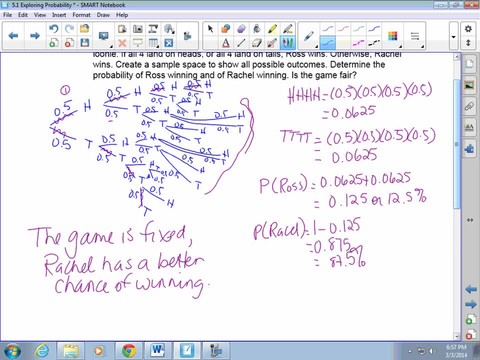 trying it out, and theoretical is when you're just looking at what are the outcomes that are possible. so that's all for the first section. good luck with your questions.